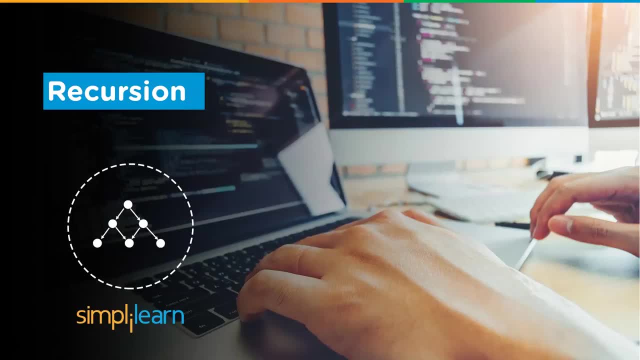 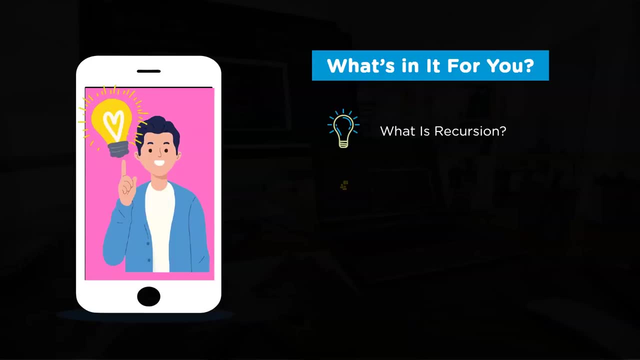 Now, without any further ado, let's get started with the agenda for today's session. We will start this session by understanding what is recursion, Followed by that, we will find out how recursion gets executed in memory area. Once done with that, we will look into different types of recursion And finally, we will implement. 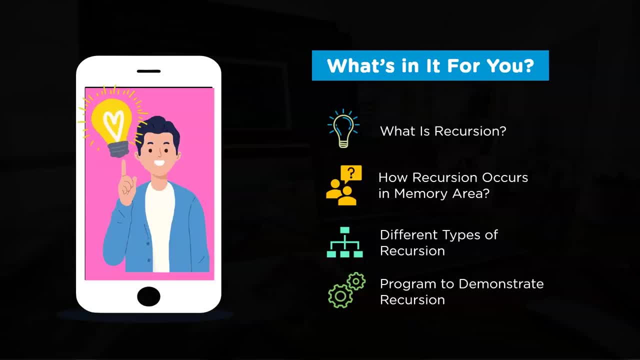 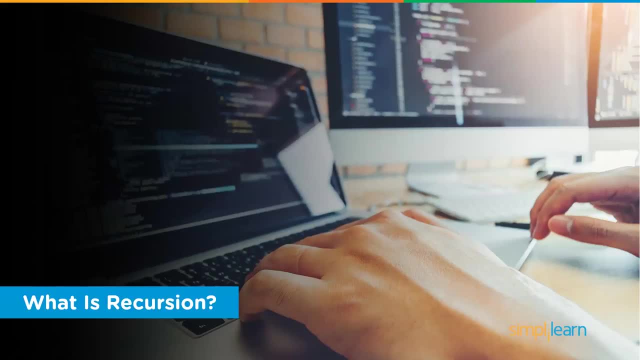 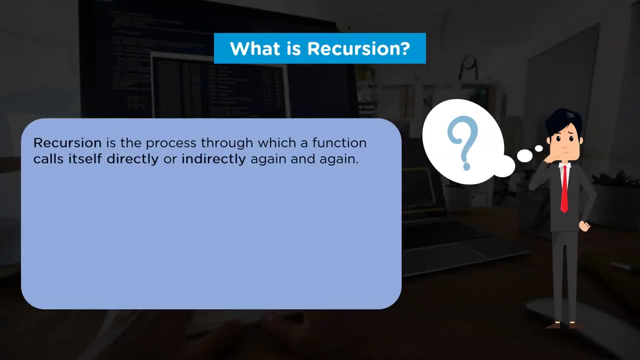 a program that demonstrates the concept of recursion. I hope I have made myself clear with the agenda. Now let's get started with our first topic. what is recursion? Well, recursion is a process in which a function repeatedly calls itself, either directly or indirectly. 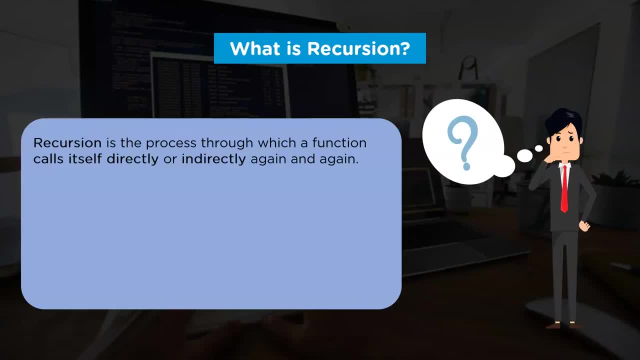 Those calls are majorly done by explicitly calling function by its name. However, it can also be accomplished by implicit calling as well. The fundamental idea behind calling the function over and over again is to break a larger problem into smaller sub-problems. We do this for reducing the computational complexity of a larger problem by breaking. 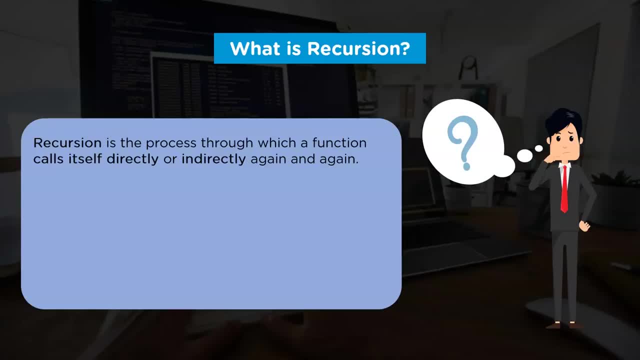 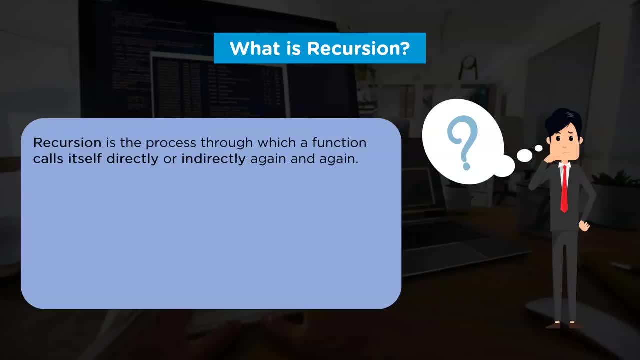 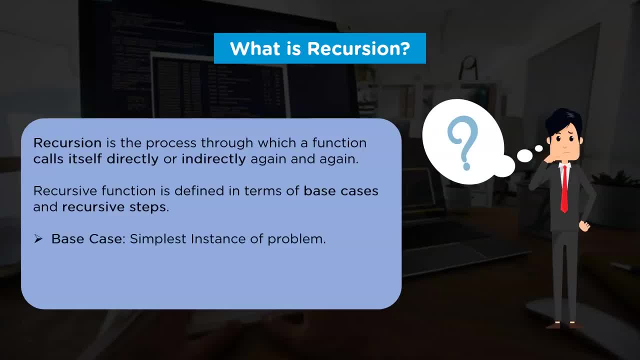 is recursive step. The base case is nothing but the simplest instance of a problem that consists of condition which holds the recursive function, Given the function calls argument, this base case computes the output of our program right away, Whereas in the recursive step, 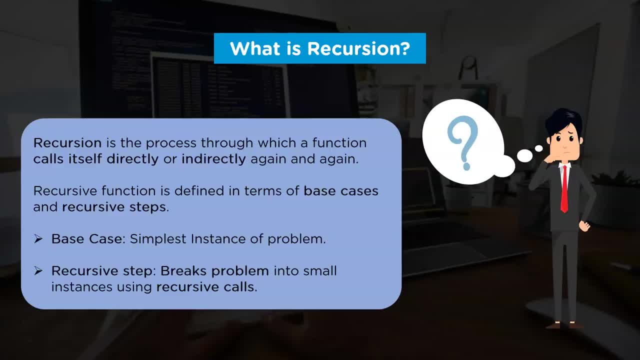 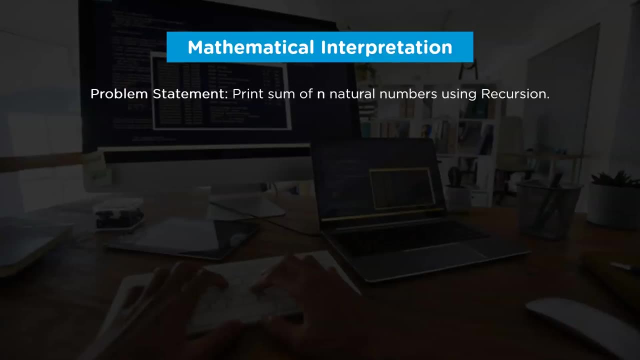 We compute the result using one or more recursive calls to the same function, but with the inputs decrease in size or complexity. To understand this breakdown, let's have a look at mathematical aspect of recursion. Suppose you have to formulate a mathematical function for computing the sum of 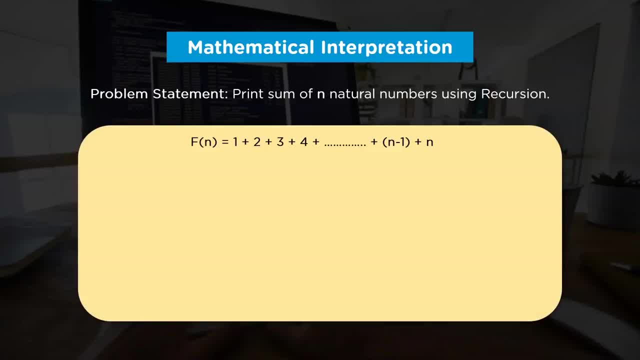 n natural numbers. That means the function that you are going to create must calculate the summation of all natural numbers in the range 0 to n. Mathematically it can be represented as: summation of all numbers: from k is equal to 0 to k is equal to n. Now the critical question here is: 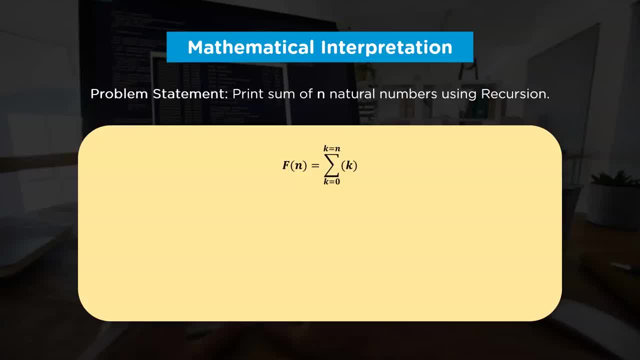 how can we actually represent this in form of recursive function? The answer is quite simple. All we need to do is break this larger problem into small fragments. We can represent this problem as: n plus sum of all natural numbers till n is equal to 1.. Now let's see how we can represent this problem in form of recursive function. 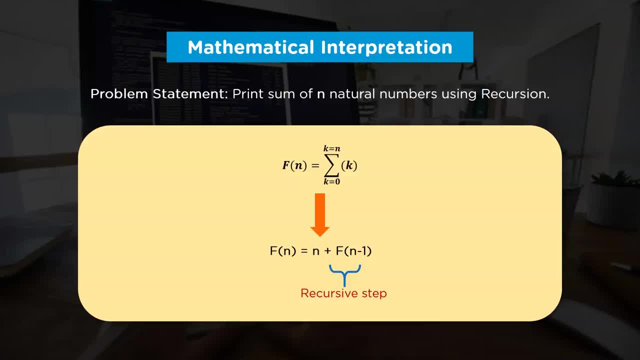 n-1.. This process of traversing in function f n-1 times is called the recursive step of our problem statement, Whereas the base case is a condition which is stopping the recursion when k is reaching value 0. In terms of programming, it can be represented using a block. Now I 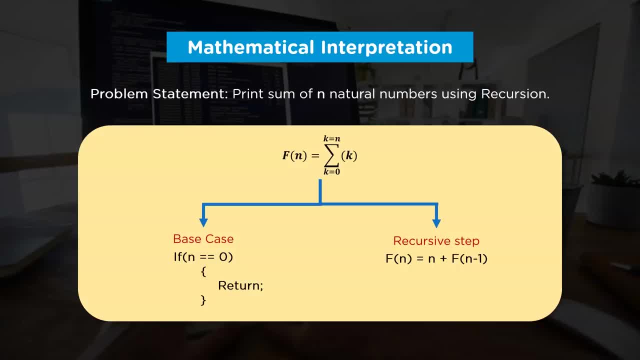 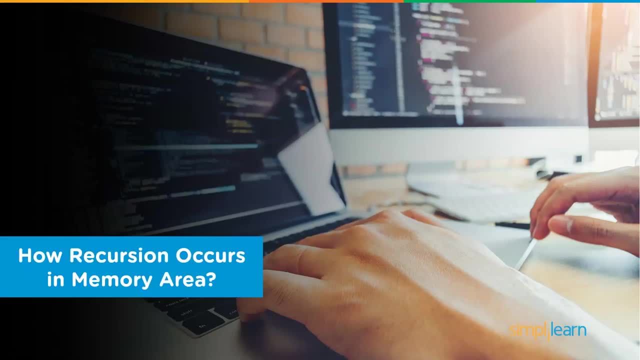 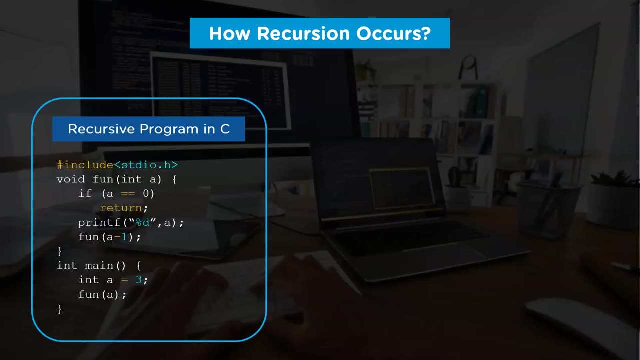 hope you guys have understood how we can break a larger problem into smaller subproblems. Moving further, we are going to understand how recursion gets executed in memory area. In order to do that, we'll take this C program as an example. In this program we have two. 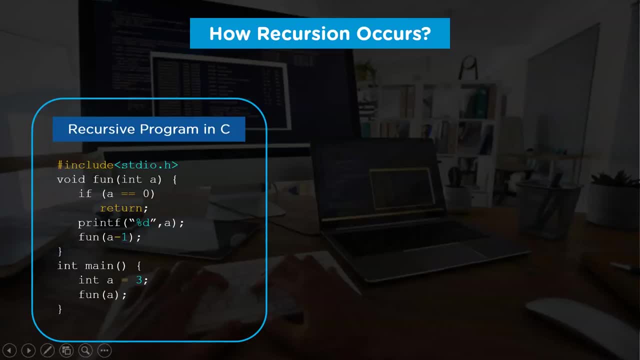 methods. The main method contains one variable and the statement that invokes a function named fun. This function, fun, is making a recursive call in its function body. We have both base case and recursive step inside this function's body. Now, whenever a function is called, its activation record will be maintained inside the stack. 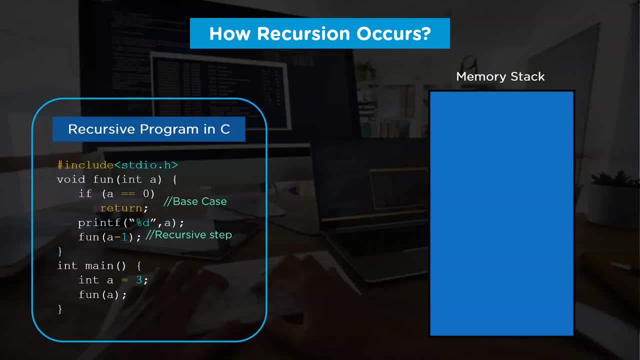 So for this program we are going to look into its control flow. As we know, the main function gets invoked primarily by an operating system. Thus we'll include the main function at first in our memory stack. This activation record will consist of local variables of 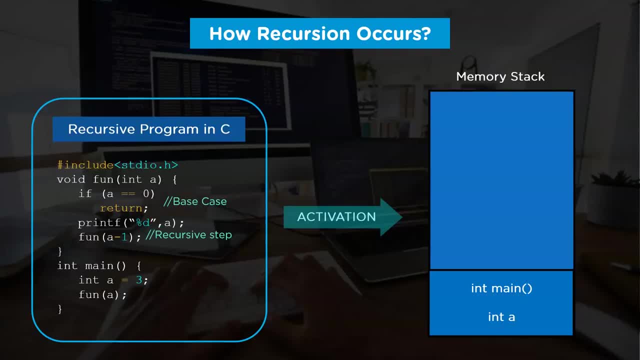 function parameters and a record of return address to the caller. But here, for the sake of simplicity, we are just not going to include the function in the memory stack. This activation record will consist of local variables, of function parameters and a record of return address to the caller. But here, for the sake of simplicity, we are just 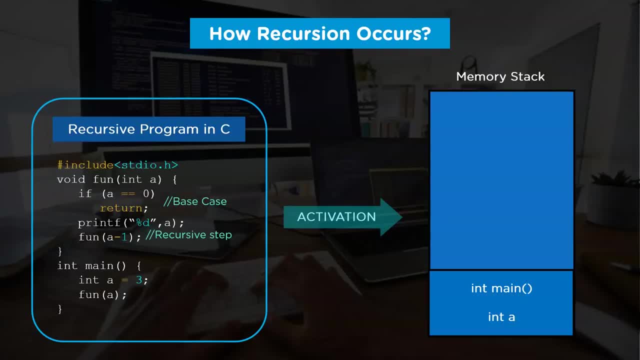 maintaining the local variables inside the activation record After this step. as you can see, the main function is activating method fun with argument 3.. Once activated, it will prompt 3 on screen and will invoke fun 3-1.. That is fun 2. Now. 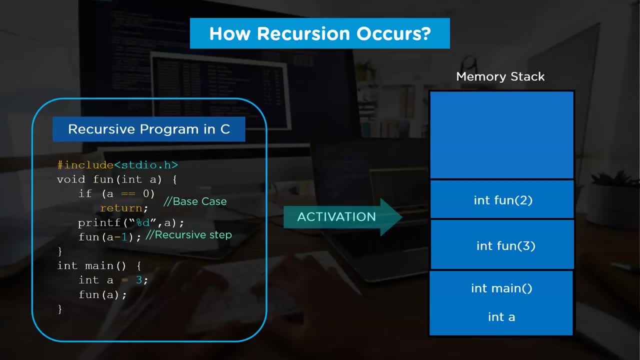 again, as 2 is greater than 0,, the control will invoke fun 2-1.. That is fun 1.. After this, the control will activate fun 0. This time, once the control enters, and if the function alters, it will execute a return statement. The activation record 0, then will get popped. 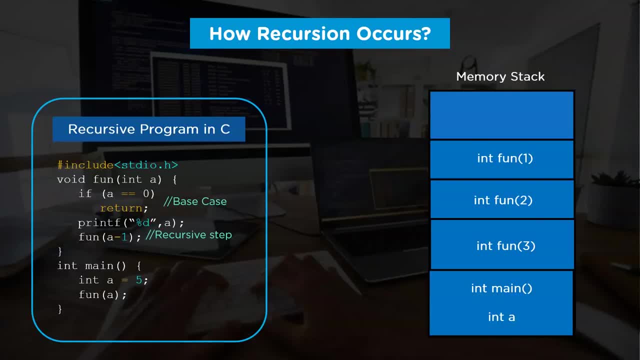 out of the memory stack. Further, every function inside the memory stack will get popped out from it, which will result in generation of output. The output that will get printed on the console for this particular program is 3,, 2, 1.. 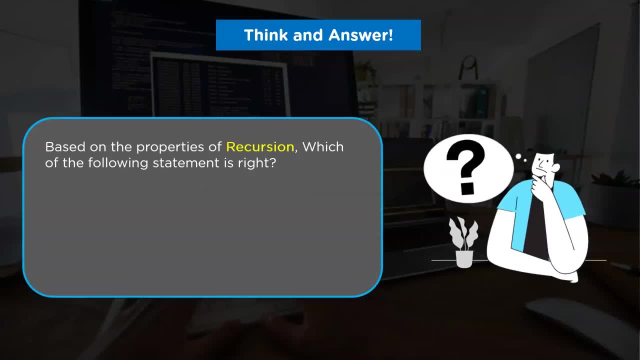 Now here is the interesting question that we want you all to answer. Based on the properties of the recursion that we have discussed till now, which of the following statements will statement seems right to you? the options that we have are: recursion is always better than iteration. 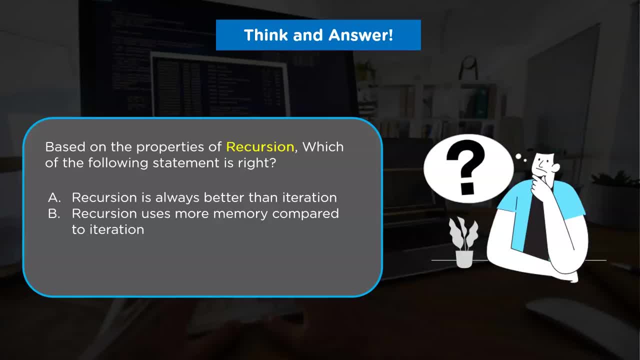 option b- recursion- uses more memory compared to the iteration. option c: recursion- uses less memory compared to the iteration. it will be interesting to see how many of you guys will get this right. so guys do leave your answers to this question in comment section below. in a week's time we'll 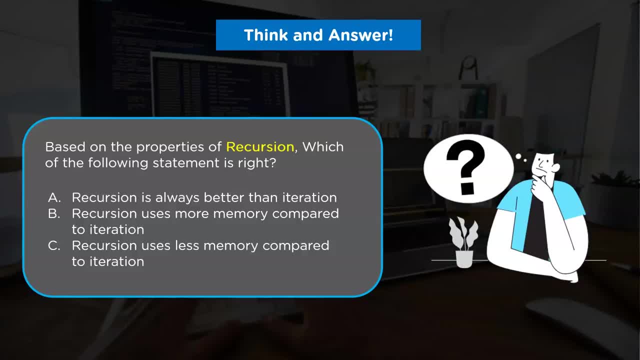 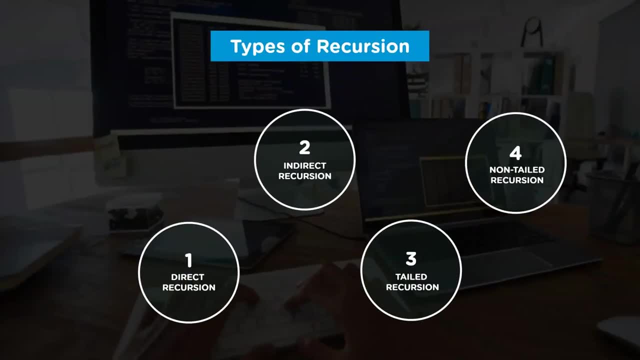 be announcing the right answer and you all can check it out. now. moving ahead, we'll discuss different types of recursion in programming. there are basically four types of recursion. the first one is direct recursion, the second one is indirect recursion, the third one is tail recursion and the fourth one is non-tail recursion. so let's discuss direct recursion. a function is: 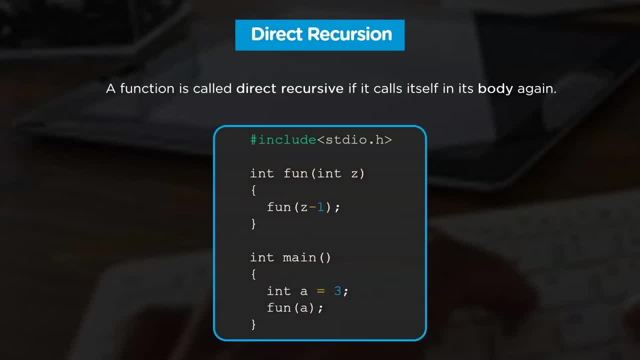 called direct recursive if it calls itself in its function body. over and over again. to better understand the function body, it is called direct recursive if it calls itself in its function body. let's look at the structure of a program that is direct recursive in nature. in this program we have: 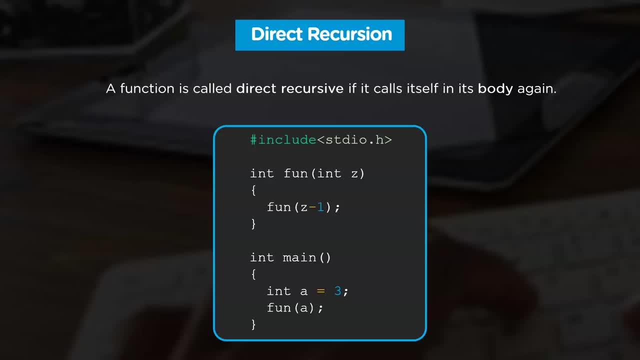 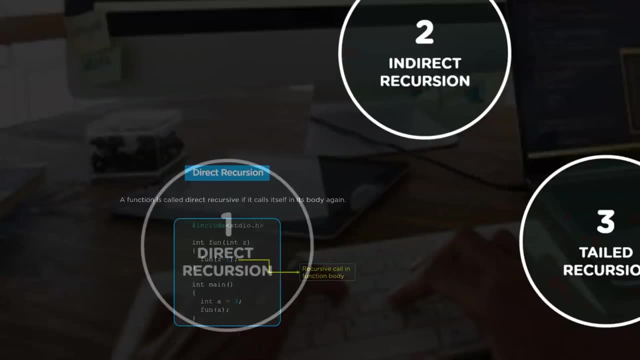 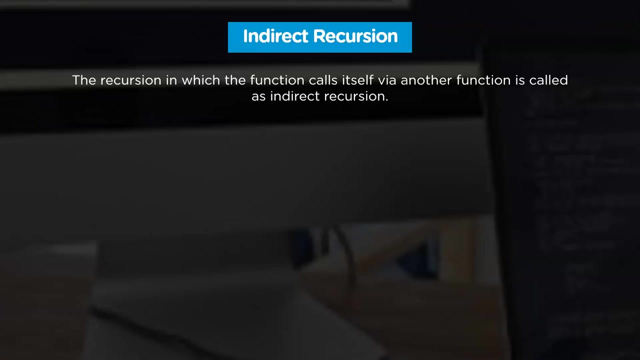 a method named fun, which is calling itself again and again in its function body. thus we can say that it is direct recursive in nature. next up is indirect recursion. the recursion in which the function calls itself via another function is called as indirect recursion. for example, in this program you can clearly see that the function fun1 is explicitly calling fun2, which 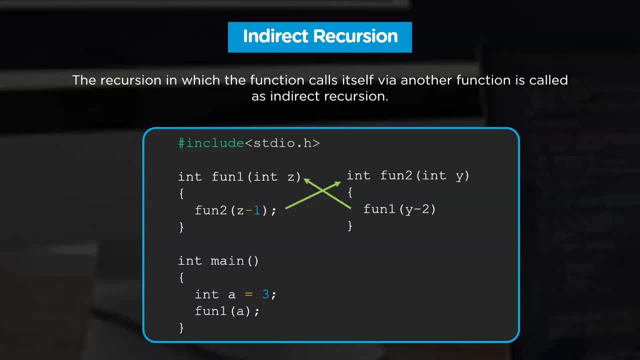 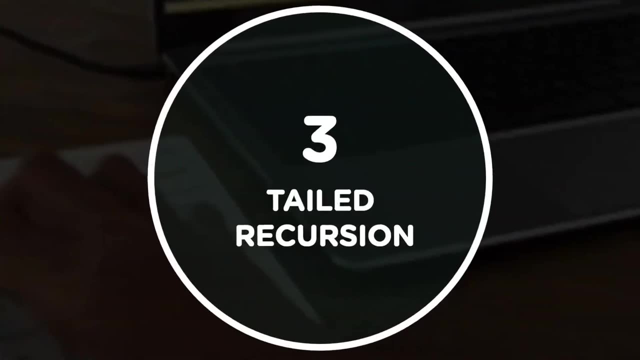 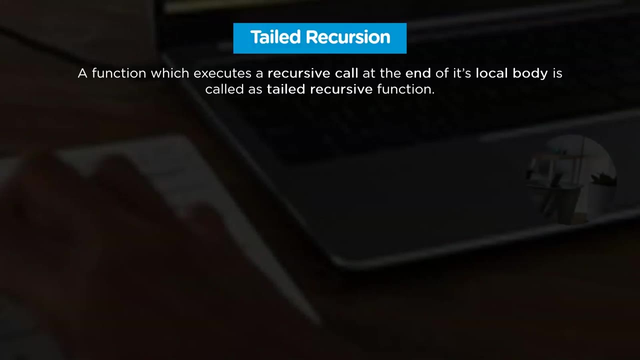 is invoking fun1 again explicitly. hence we can say that this is an example of indirect recursion. further, we have tail recursion. a recursive function is said to be tail recursive if the recursive call is the last execution done by the function. let's try to understand this definition. 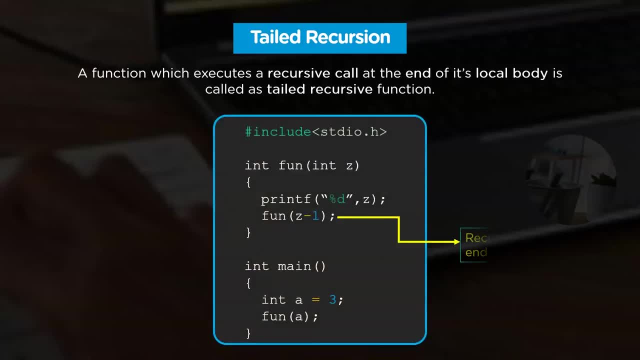 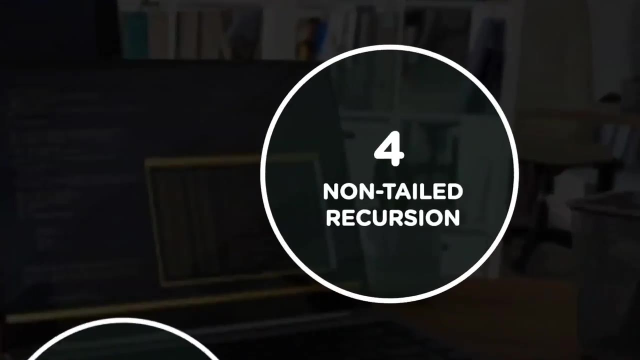 with the help of an example. if you observe this program, you can see that the recursive call is the last line adi will execute for. method fun is recursive call and because of that there is no need to remember any previous state of our program. finally, we have a non-tail recursive function. 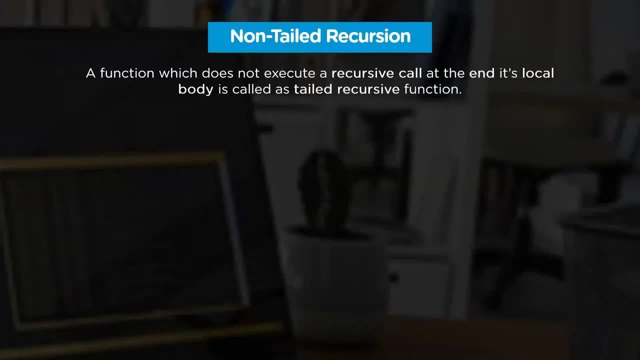 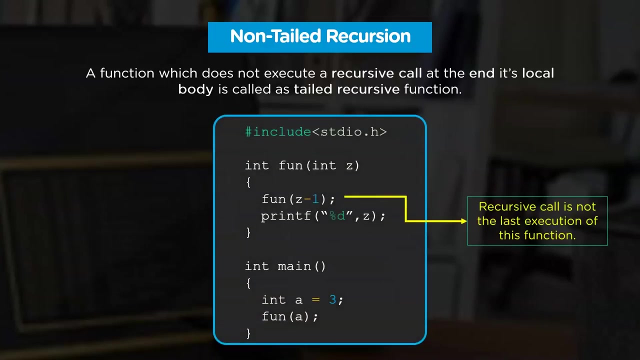 on our list, a recursive function is said to be non-tail recursive. if the recursion call is not the last thing done by the function after returning back, there is something left to evaluate. let's consider one example. in this function, you can clearly observe that there is another operation after the recursive call. hence our adi will have to. 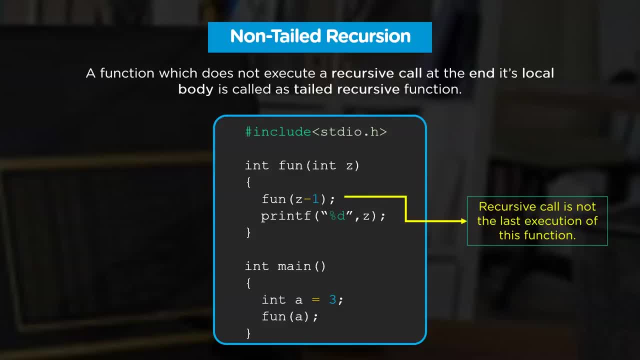 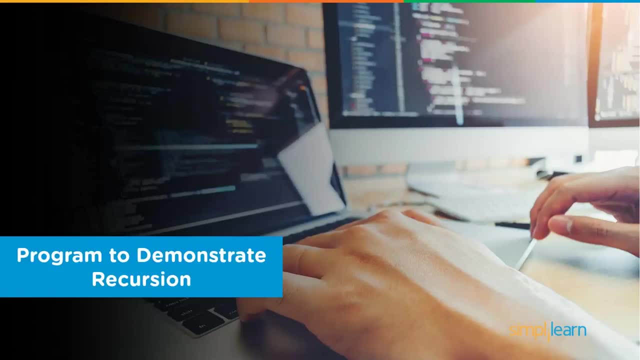 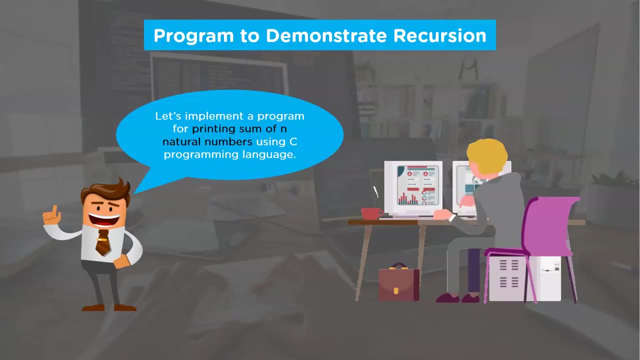 memorize the previous state inside this memory block. that is why this program can be considered as non-tail recursive. now, finally, let's implement a program to demonstrate the recursion, the program that we are going to implement its solution to the problem statement that we discussed earlier. 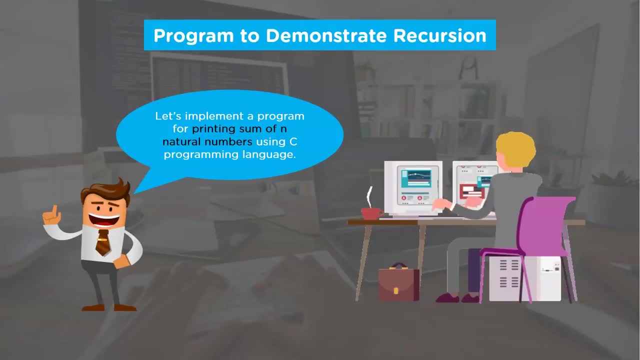 according to that problem statement, we have to calculate the number of recursive functions in the argument and we have to calculate the sum of n natural numbers, given the number n. now, in order to address this problem, we are going to use c programming language, so without any further ado, 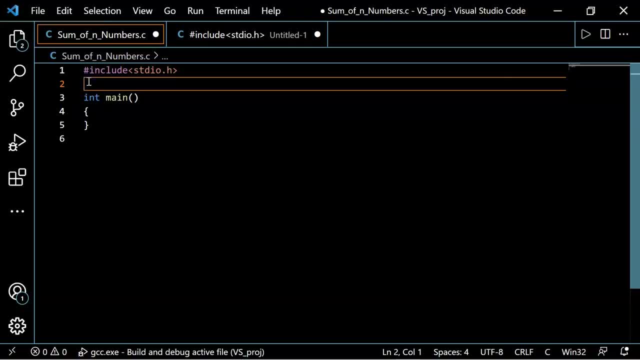 let's head over to the code editor now in order to get started with coding implementation. first we'll create an utility function to calculate sum of n natural numbers. so let's do that and we'll pass an argument and n. now we have arrived inside the body of function sum. what we'll first do is we'll calculate sum of n. 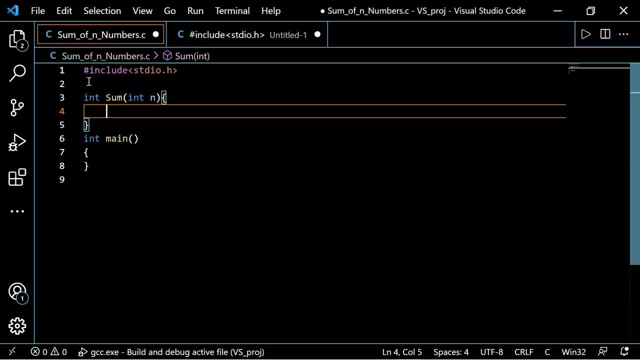 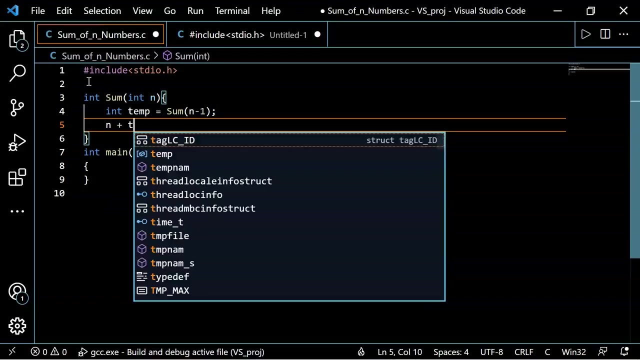 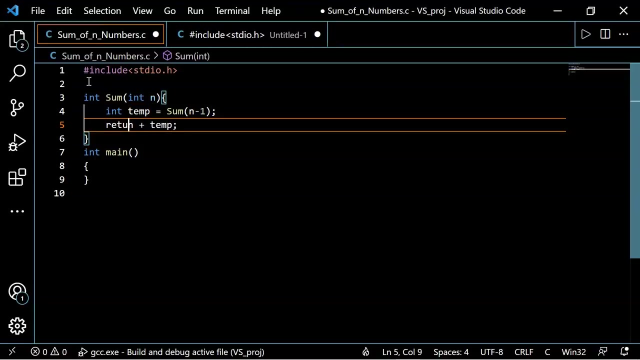 minus one natural numbers by making an recursive call to function sum. so let's do that: sum n minus one and we'll store this value inside temporary variable. now we'll add this temporary variables value in order to return it. as an result, the statements that we just wrote are called as recursive steps, but if you observe the statement, 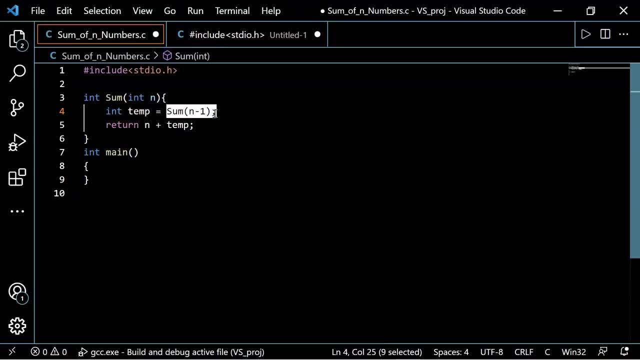 we are not putting any limitation to our recursive call, so that is why we'll have to add base case to our function. so let's do that: f? n equal to equal to zero, then return zero. with this, we have successfully implemented our sum function, so let's work on our 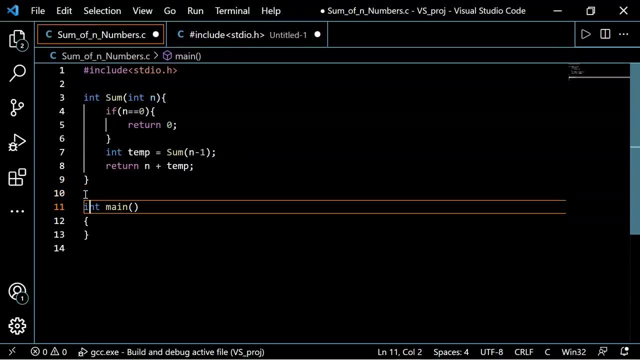 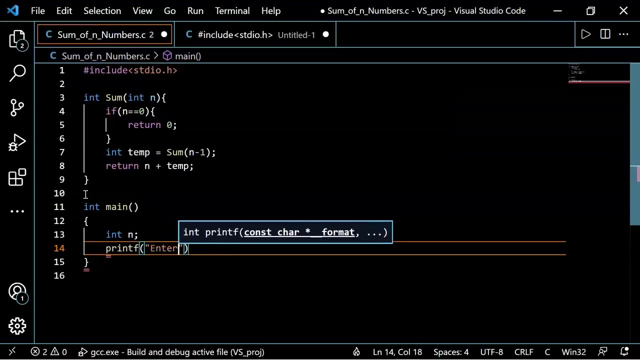 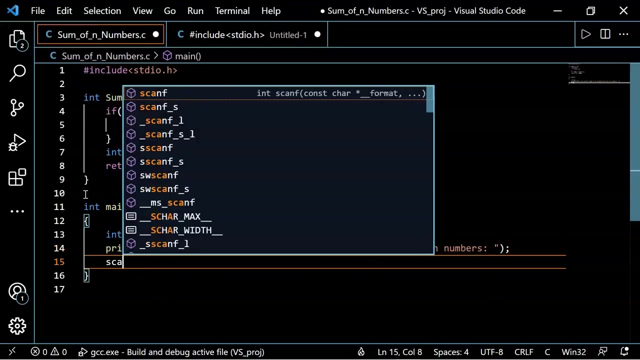 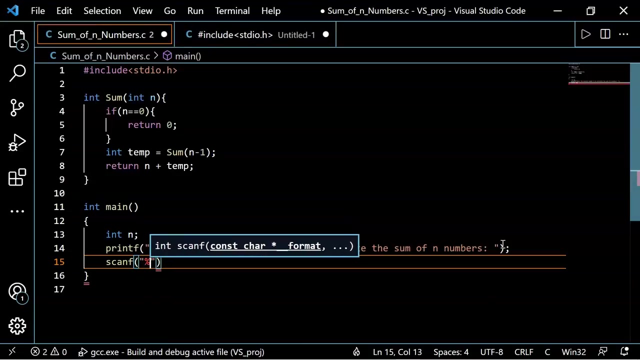 driver method. to generate the result in this driver method, first we'll create an variable n and after that we'll write a printf statement, enter the natural number n to calculate the sum of n numbers, semicolon, and in next line we'll write scan up statement in order to take input from our user. so inside this we'll write modulus d. 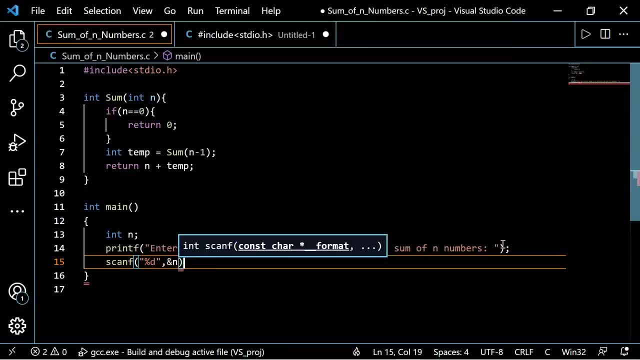 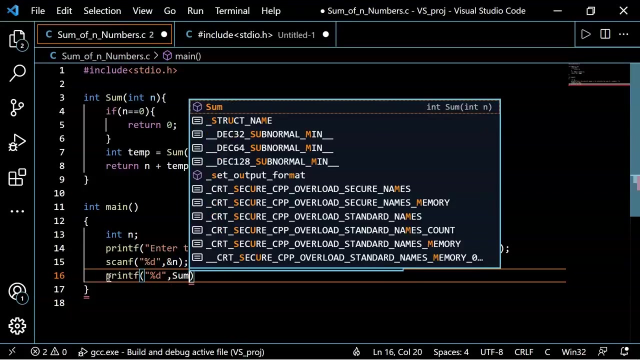 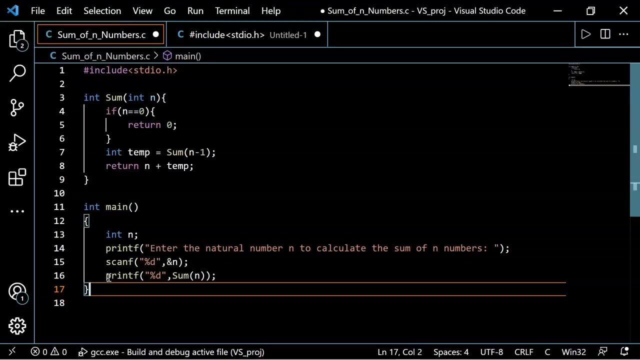 comma, ambracin, n and semicolon. and in next statement we'll make a call to our sum function in order to calculate sum of n natural numbers. so how we can do that? well, we can add modulus d here, comma, sum n, semicolon, and i hope our code works fine now. so let's check it by compiling.